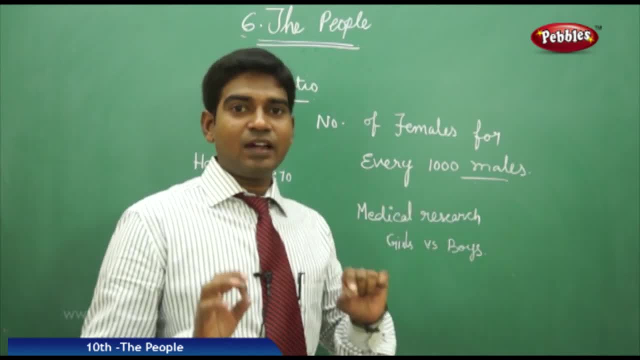 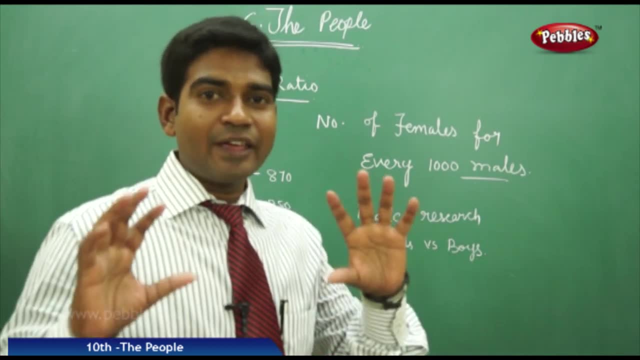 What would be the reason? But according to the medical facts, it is clear that girls can survive better than boys. So it is only clearly evident that there is discrimination. in our country We are experiencing the discrimination. The girls who are medically fit and fine are not. 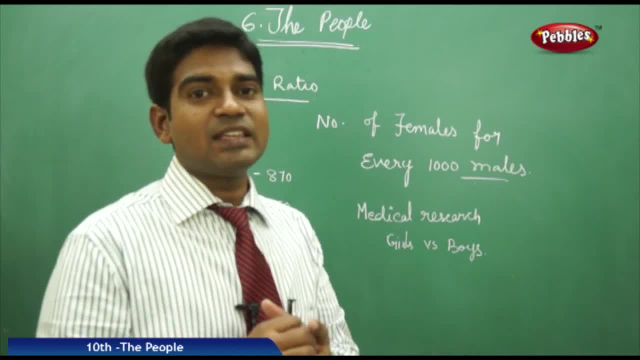 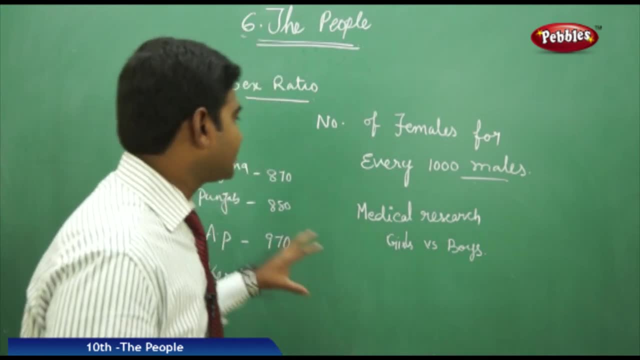 provided any proper care for them so that they are not able to sustain that one and they are losing their lives. This is one of the basic reason what we are having the negative impact on our lives. If you see the state's comparison for us in Haryana we have, for every 1000 males, 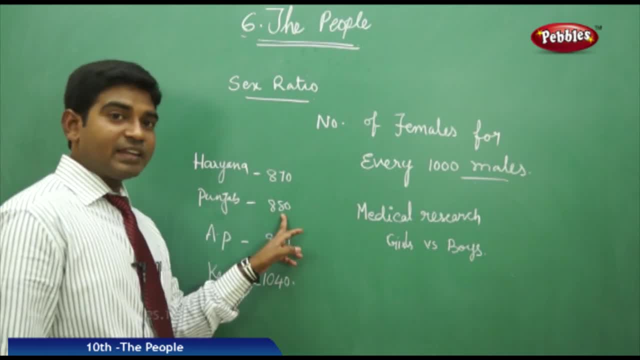 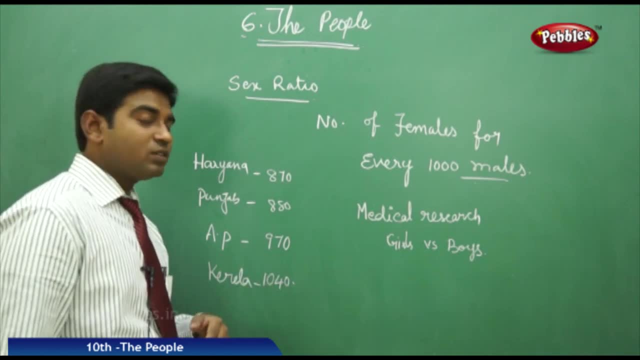 only 817 girls and in Punjab we have 880 for every 1000.. APV is better- 970, and Kerala- it is fantastic, Like above 1000, we have 1040 females surviving here, So where there is a proper. 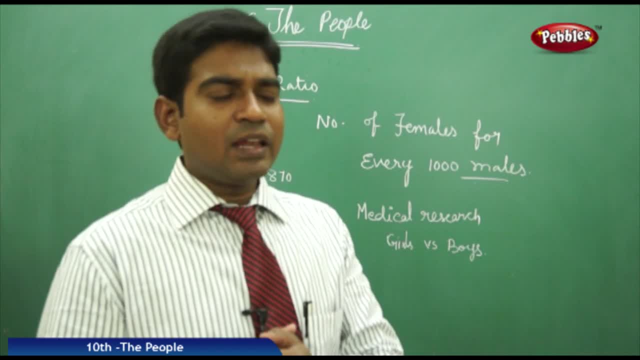 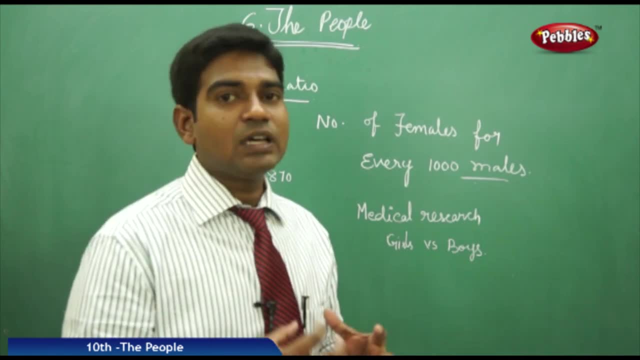 education and understanding. then we can have the proper issues there, Like in a family when if there is a girl and a boy, a brother and a sister, the utmost care is taken for the brother when compared to the girl sister. Sister is having an issue here. She is forced to work at home. She is 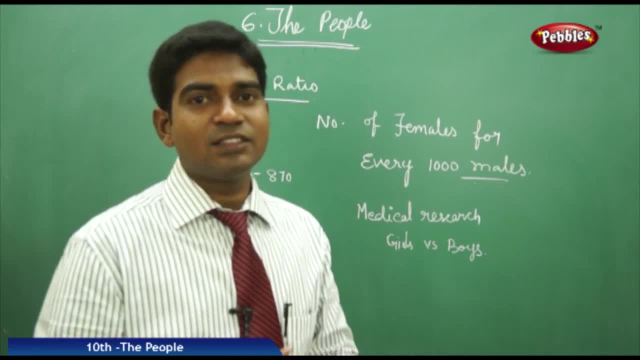 not allowed to send her husband, She is not allowed to send her husband, She is not allowed to send her daughter to high school, or there are some biases regarding this issue. So it should be addressed very carefully and education has been a major relieving or discriminating factor to come out of. 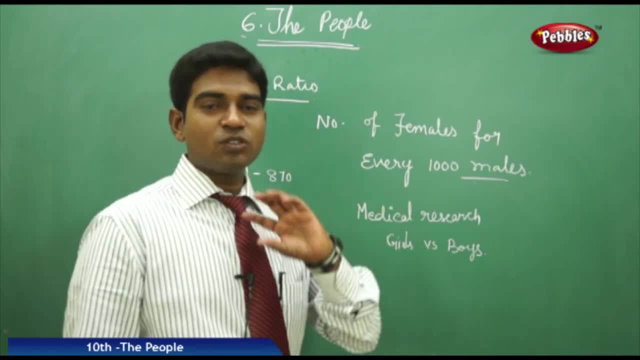 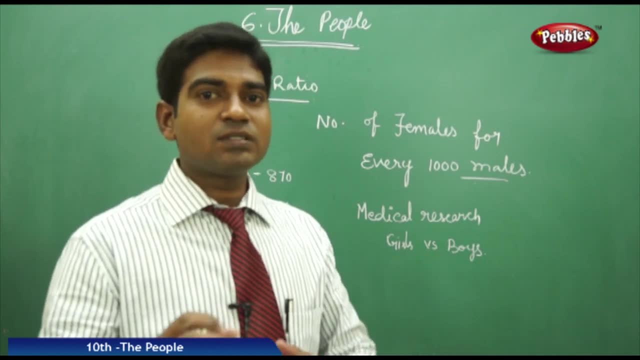 the girls' interaction of all these kinds of issues and all these things, Because once the girls and boys are educated, we can have an equal opportunity for them. Even girls are also able to better than do boys, because they are able to do the homework as well as they are able to do the household works. 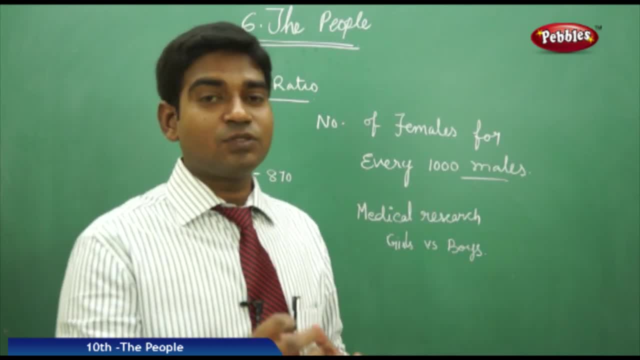 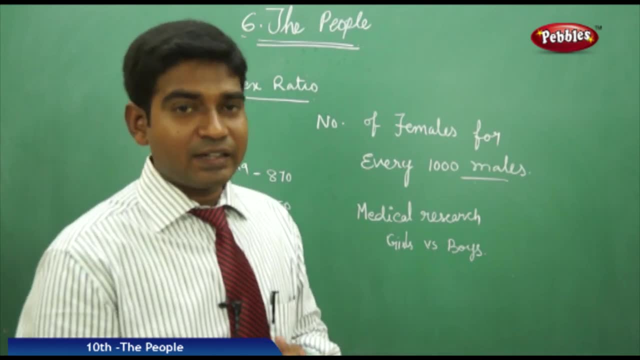 and now we are having many entrepreneurs who are working successfully managing both professional things. So the sex ratio is a serious issue. It has to be addressed in India in the context, especially when, compared to, the sex ratio means the females for every 1000 males, and the medical researchers have 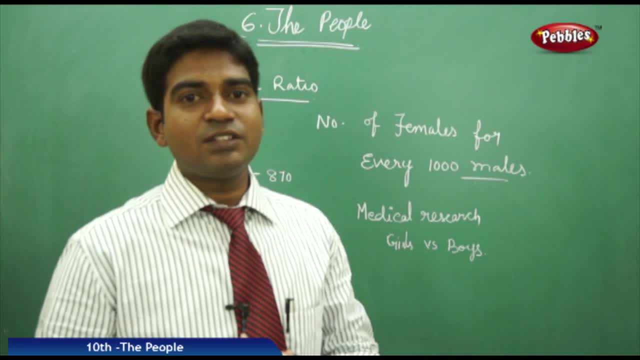 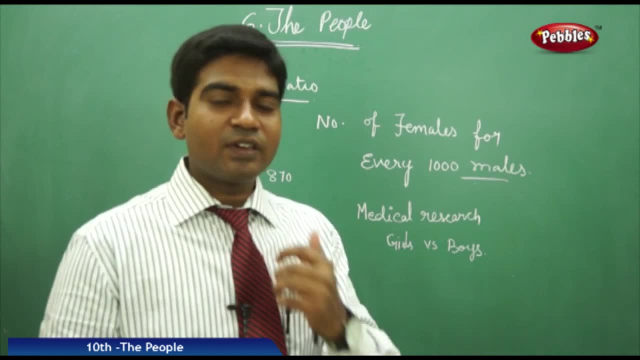 proven that girls are better than the boys. So let us understand the issue that there is no discrimination should be understand here. like boys and girls- Both are children- should be taken care properly. Then only we can reach to the height of our success. Education could be a key progress to change the issues Like in: